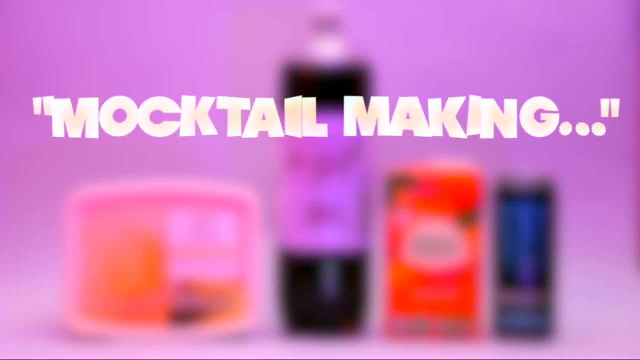 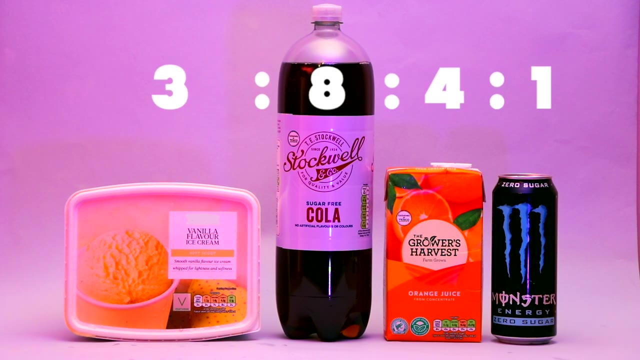 In another example I read about a great recipe for a mocktail that I want to try out for a party. The recipe tells me I need 3 parts ice cream to 8 parts coke to 4 parts orange juice to 1 part an edgy drink. 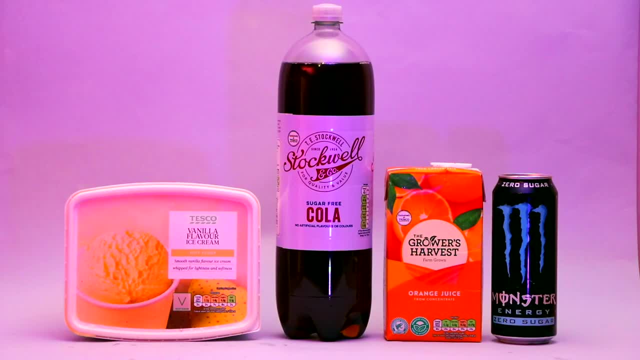 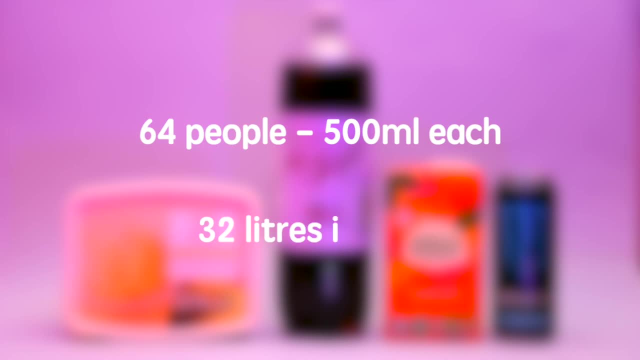 Sounds delicious, Looked great, tasted great. I'm looking to make enough for at least 64 people to have one 500ml drink each. That means I'll need to make at least 32 litres of this mocktail, But there's a bit of a problem. 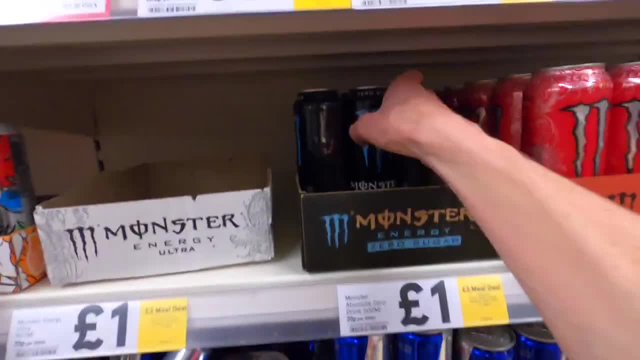 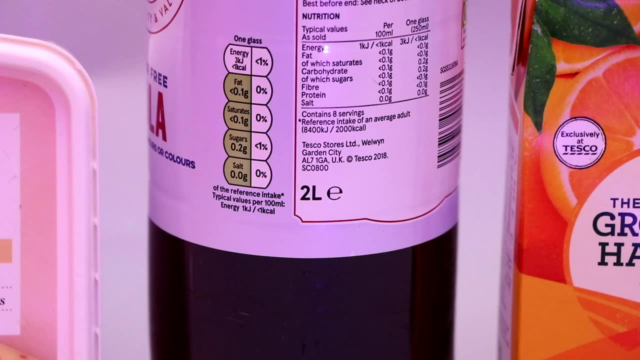 When I was in the shop, I noticed that all the container sizes are different for each ingredient. The energy drinks come in cans of 500ml, The coke comes in 2 litre bottles. The orange juice comes in 1 litre cartons. 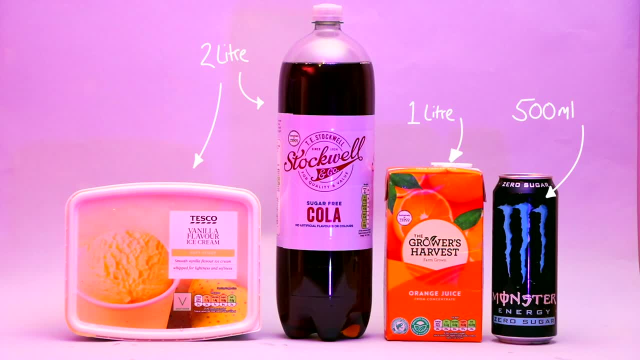 And the ice cream comes in 2 litre tubs. So let's do some calculations. If we say that the energy drink, which is 500ml, equals 1 part, that means both the coke bottle and the ice cream, which are 2 litres, would equal 4 parts. 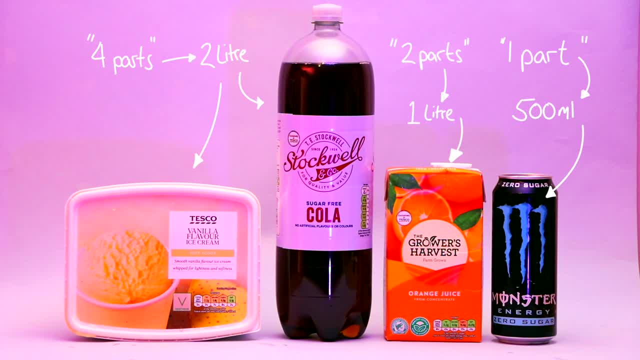 While the 1 litre carton of orange would equal 2 parts, Make my ratio of 3 to 8 to 4 to 1.. That would mean that I would need 1 can of energy drink to 2 bottles of coke. 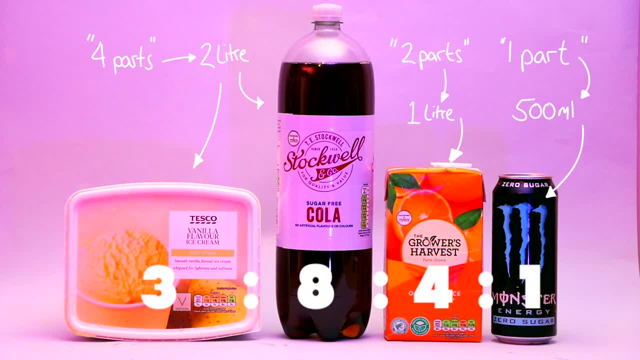 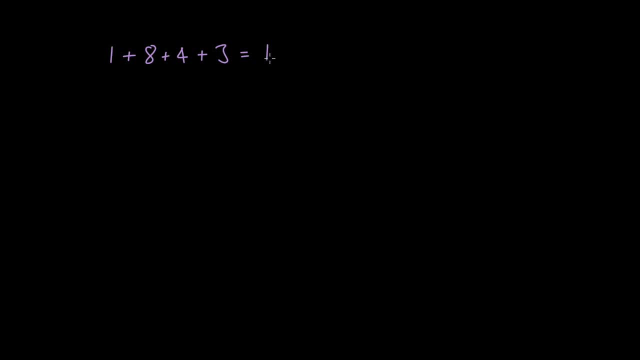 to 2 cartons of orange juice, to 3 quarters of a tub of ice cream. Hmm, With the numbers in my ratio, where each part equals 500ml, I have 1 plus 8 plus 4 plus 3,. 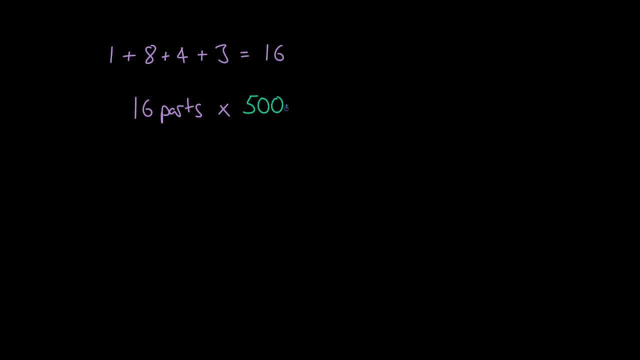 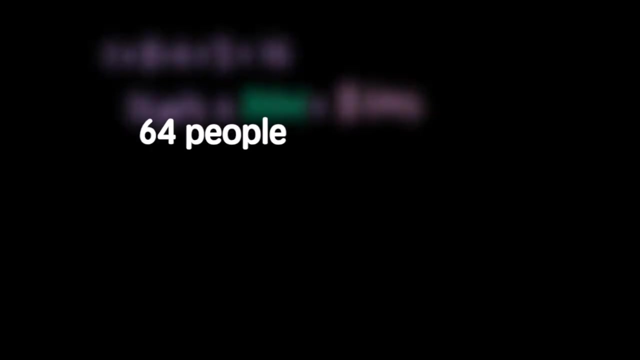 totaling 16 parts. 16 parts times 500ml will give me 8 litres of this mocktail. I know I have 64 people coming who all want 500ml each And, as we've already said, I'm going to need 32 litres in total. 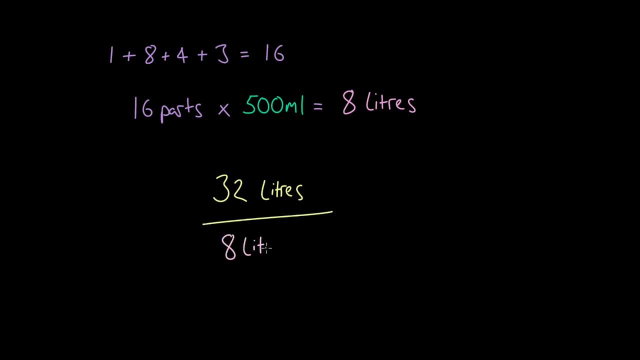 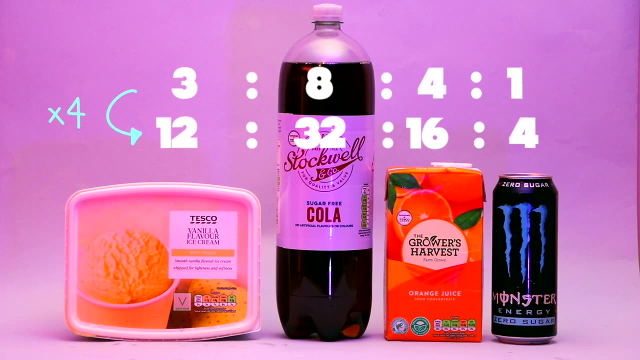 8 litres divides into 32 litres exactly 4 times. So that means I need 4 times as much of every part. The ratio by 4 means I need 4 parts energy drink, 32 parts coke, 16 parts orange juice. 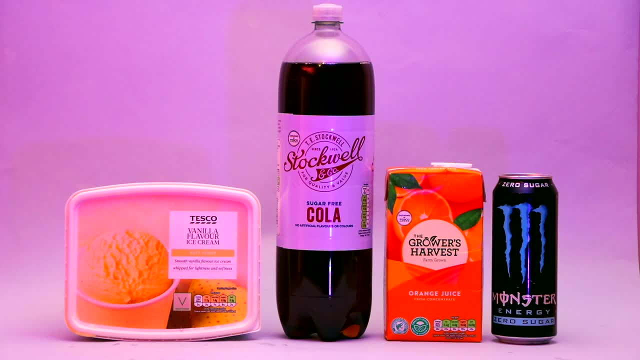 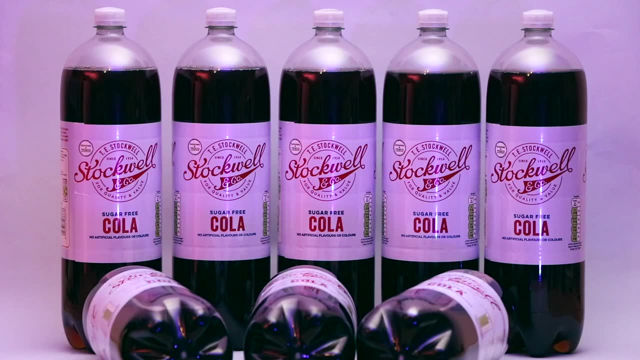 and 12 parts ice cream. Thinking about this ratio in relation to our package sizes, our final shop would then require 4 cans of energy drink, 8 bottles of coke, 8 cartons of orange juice and 3 tubs of ice cream. 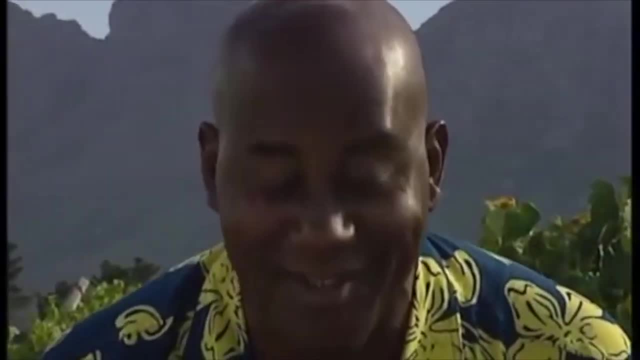 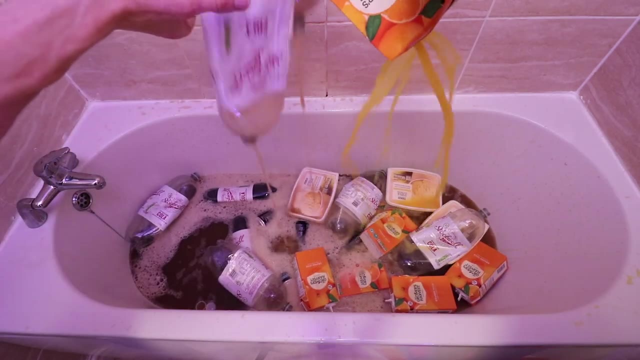 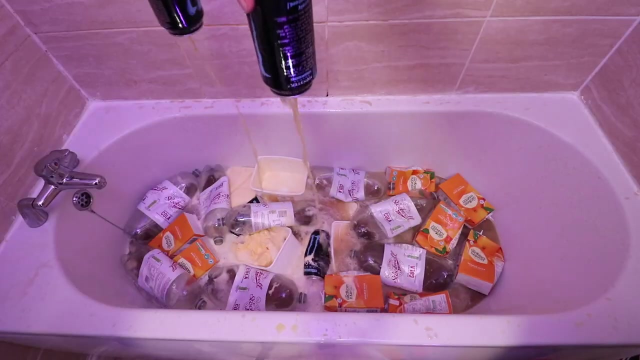 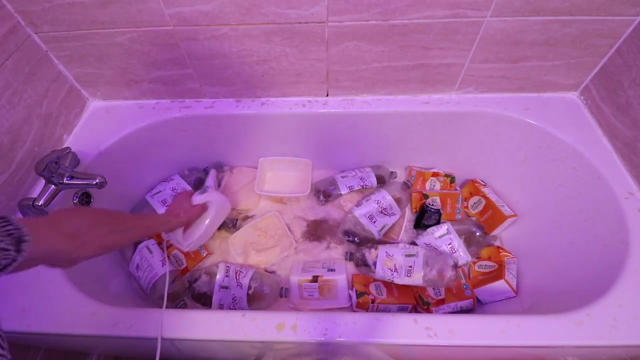 Delicious, So attractive And, believe me, it tastes magnificent. It's a lot of fun. It's a lot of fun. I mean, Wow, It's a lot of fun. We are talking too. Oh Look, great Tasted great. 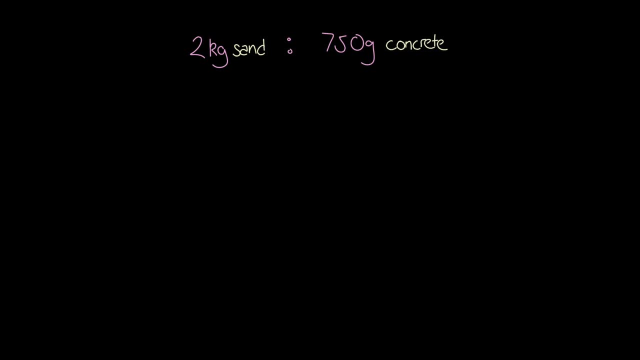 Get the old eyes going In the final part. let's take a quick look. I've been given the ratio of 2kg sand to 750g concrete for a cement mix and I want to find the simplest ratio for a bulk order. 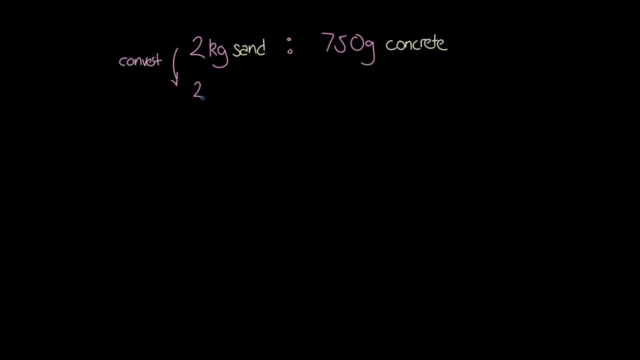 First we need to convert the 2kg into grams, giving us 2000g in total. Then we can begin to split 2000 into its prime factors. 2000 can be divided by 2, giving us our first prime factor. 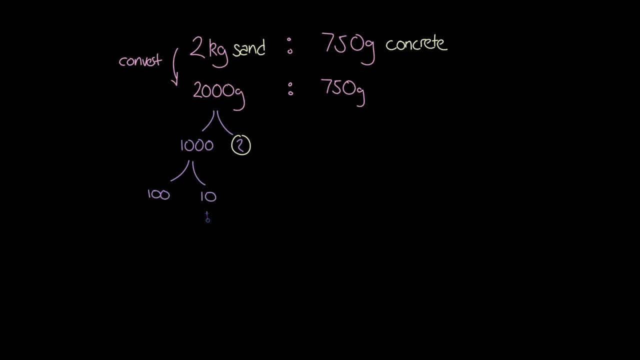 1000 can be split into 100 times 10. This 10 gives us two more prime factors of 2 and 5.. And similarly, we can split 100 into two 10s, which then both divide down into 2 and 5.. 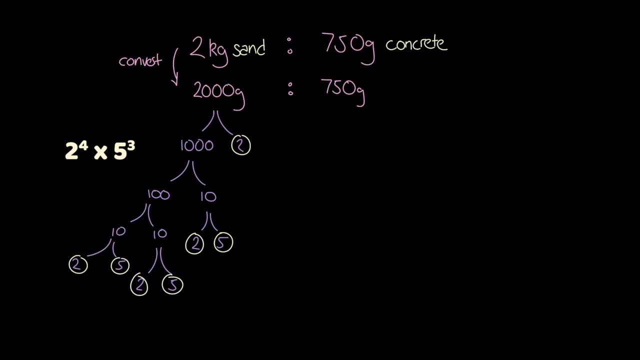 So our final prime factorisation for 2000 is 2 to the 4th power times 5 cubed. Rising through the same process for 750 gives us our prime factors of 2 times 3 times 5 cubed. Taking out factors that occur in bulk gives us the highest common factor of 250. 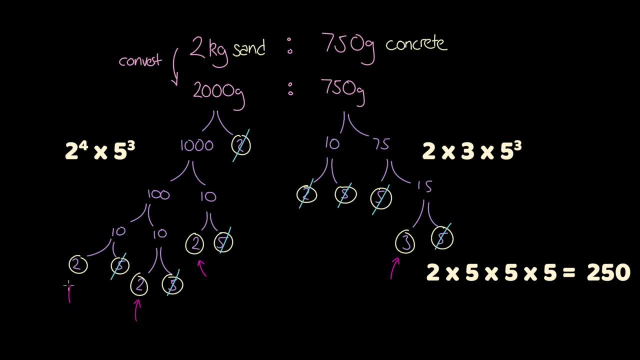 This means that what we have left is a prime factor of 2 times 3 times 5 cubed, And what we have left is the lowest factor in each part of the ratio that isn't common with the other. So the simplest form of our ratio. 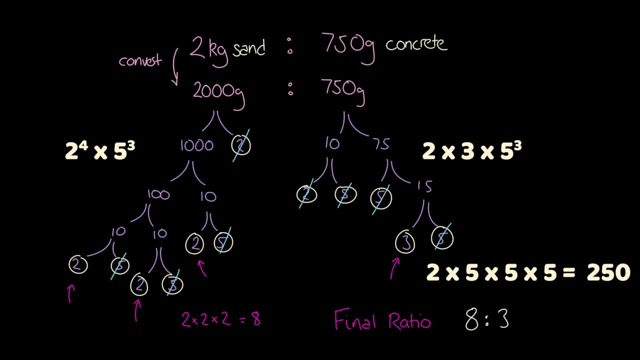 And that's it. Thanks for watching and I hope this has helped get your head around some ratios more easily.